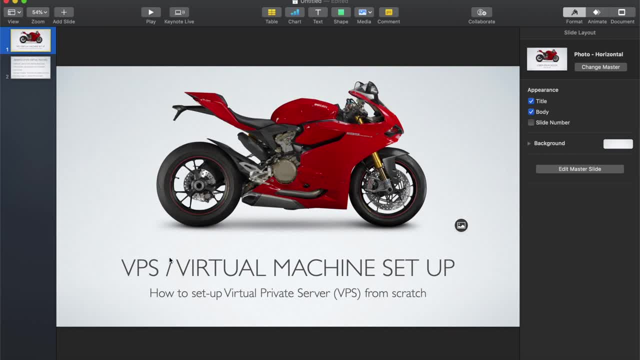 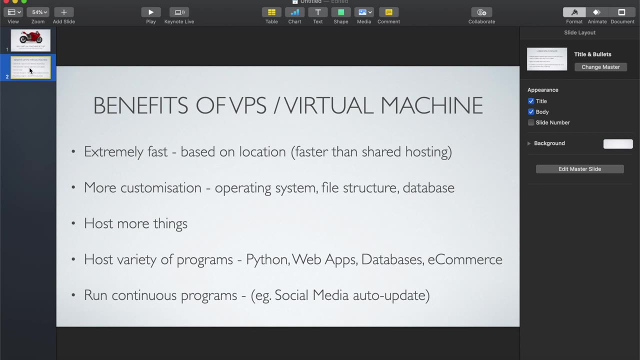 let's just go through. um, first of all, we are talking about the vps, which is a short for a virtual private server or a virtual machine. okay, so, um, why would you want to use a vps or a virtual private server? the first reason why i personally like to choose them is that they are usually 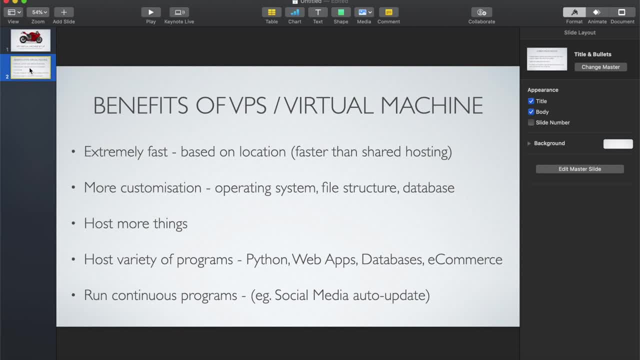 a shared service. so if you're trying to host a website, for example, you could either go for a shared- um you know, a shared computing, or a shared server where you are hosting the machine with other people sharing the same ip address, but that is usually um a bit slower. 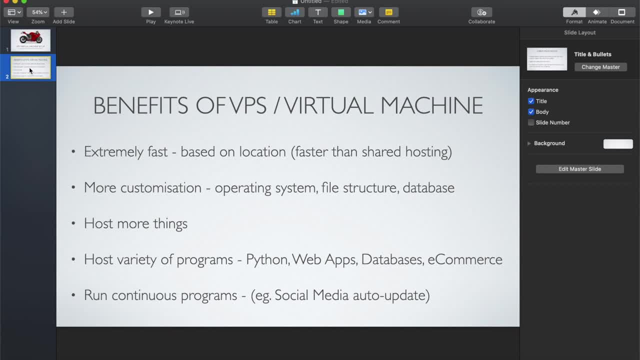 and um, you know you can't configure much. you you basically can only do. you know what you are available to, what's available to you based on the operating system that the shared server is working with. but if you create your own private server, you could set it up there. 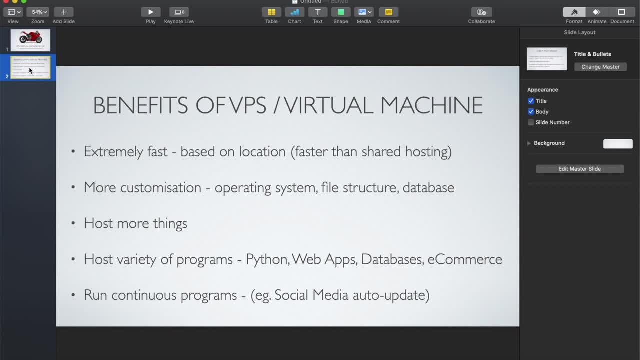 that you want from the operating system upwards. um. the second thing is that obviously you have more customization. you can pretty much put whatever operating system you like file structure, which enables you to do a whole lot of complex tasks you would not be able to do with shared hosting. 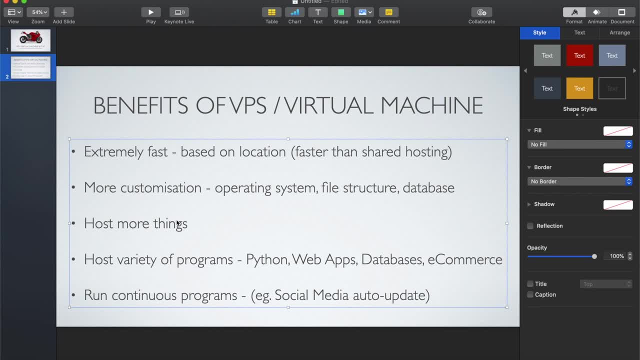 you can host more things. okay. you can host a web application. you can host a database. you can host even an e-commerce website. you can even host a wordpress website. you can host even multiple sites- up to a hundred websites, depending on the size of the vps- okay, so you can do multiple things with it. 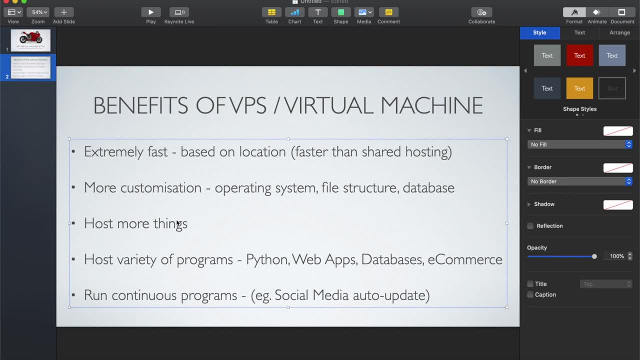 that you wouldn't be able to do with shared hosting. and the last one is: you can run continuous programs, and so the second part of this tutorial will be when i'm showing you how to um run a python program on a vps that's going to be running continuously, day and night, whether you're awake. 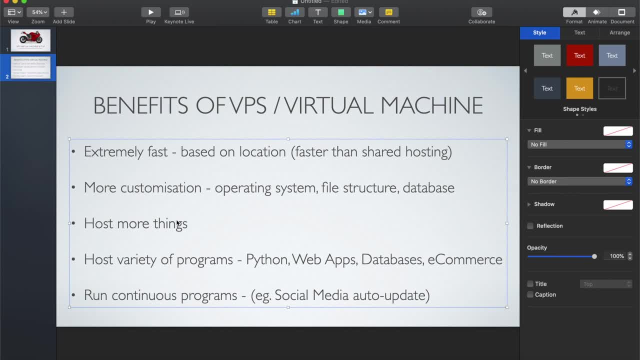 whether you're sleeping running on the vps, and you can only do this on a vps. so that's one of the things i love about about this machine. so let's get started. so let's get started. so let's get started, get started. so get over to your internet explorer and um, let's search for. um, we're gonna, let's do a. 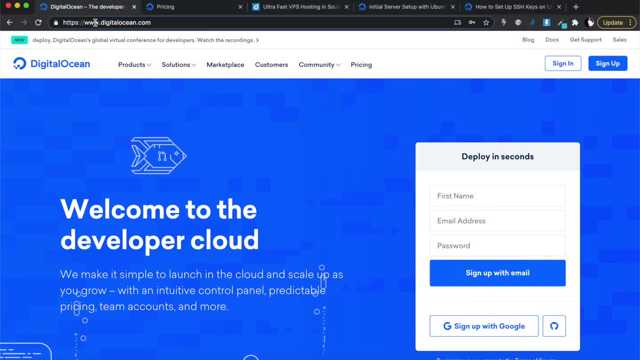 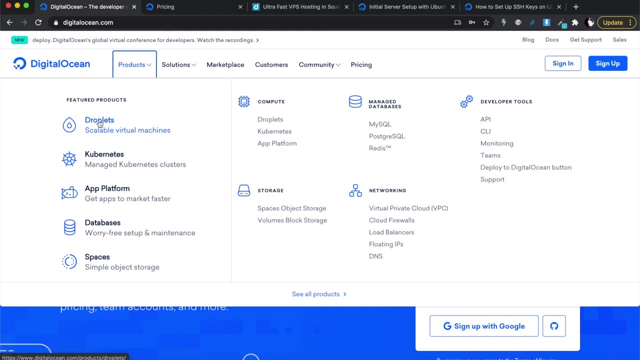 quick comparison first. so let's start on digital ocean. so just go to wwwdigitaloceancom, all right. and then under products, yes, i know, and the products, let's um click on droplets. okay, so they call their virtual machines or the vps- virtual private servers are droplets, but 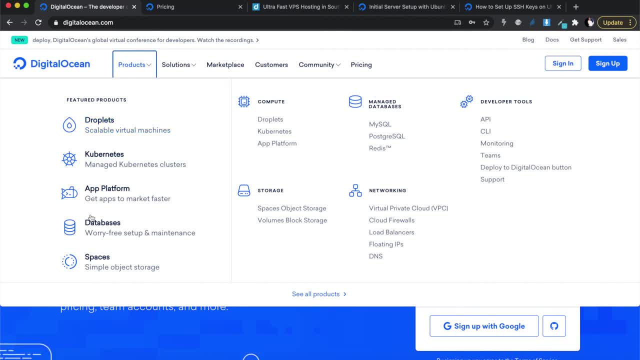 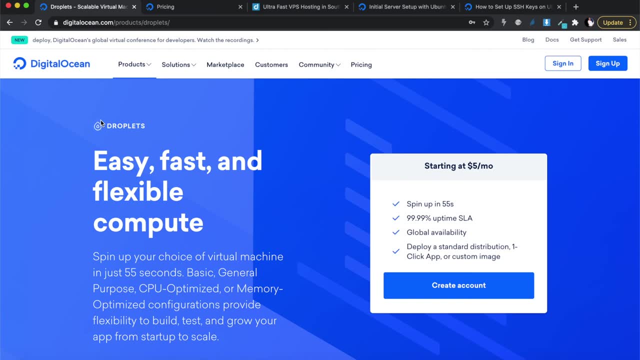 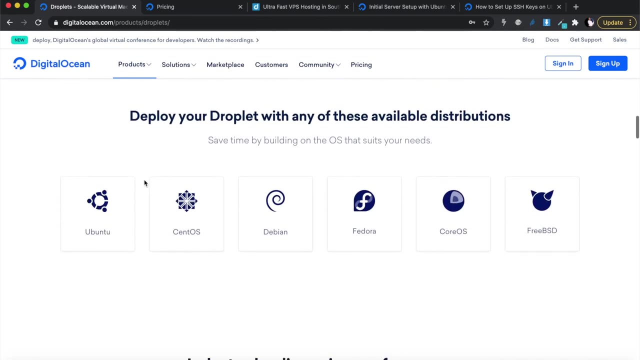 it's basically the same thing. they have a lot of other services that they offer here, guys and um. you won't have time to go through all of it today, but let's just focus on the droplets and um. so go through this and read it right. so this is what um they offer in terms of droplets, and you can see. 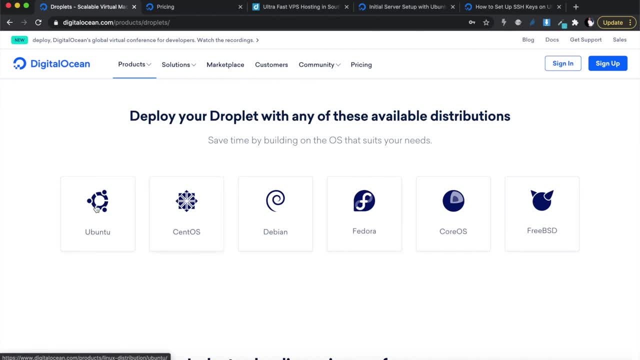 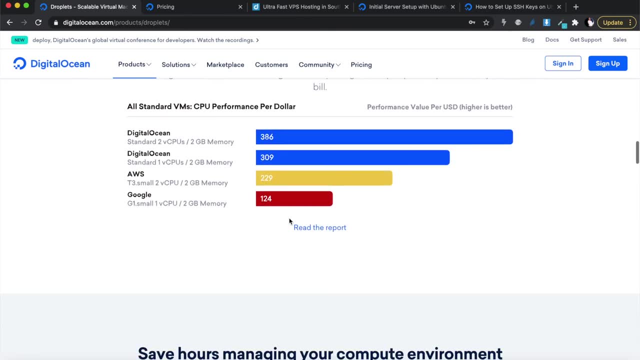 the operating system that they offer. you can install anything from ubuntu to debian to fedora. it's really up to you depending on what you're going to be using this droplet for, all right and based on um. you know the industry standards. you know there's a lot if you want to sort of go. 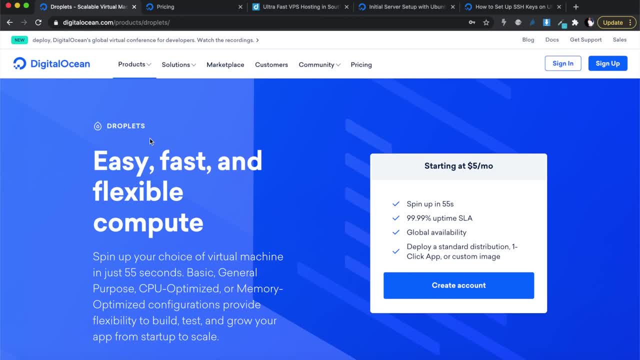 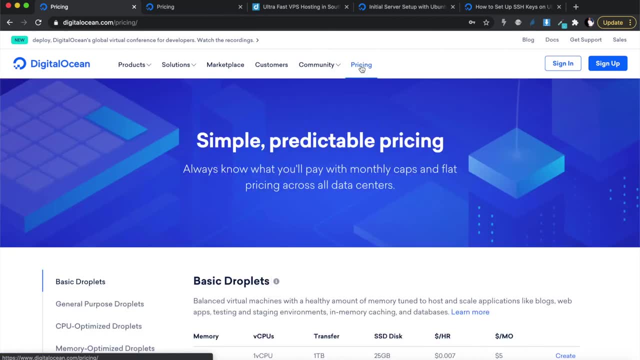 through what they're offering that you can read through here on digital ocean. but i want to just show you quickly the pricing and why a vps actually offers you better value for money if you're not willing to get your hands- i mean if you're not afraid to get your hands dirty- so the cheapest. 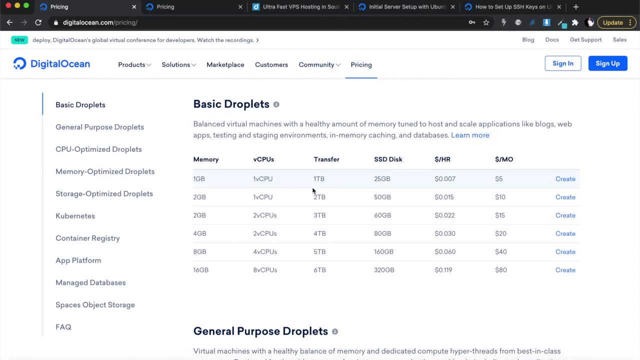 vps that they've got. is this one gig um, one cpu, uh, one terabyte transfer, that's 25 gigs of space- only going to be paying five dollars for this a month. i did a quick calculation. five dollars is approximately, currently, with exchange rate in south africa, about 80 rand. all right, so i'm going. 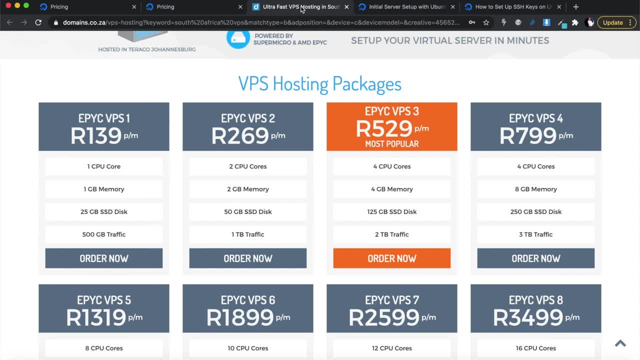 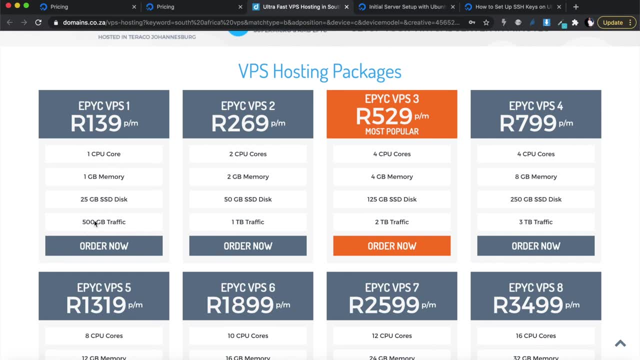 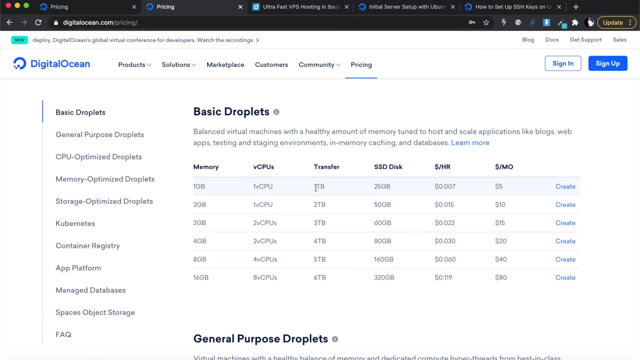 to compare this with the best, i believe, south african hosting provider, which is w2c, and look at a similar package. okay, one cpu call, one memory, um, actually this 500 gig of traffic and this one here is is one terabyte of traffic, so actually they've got a better deal on um. 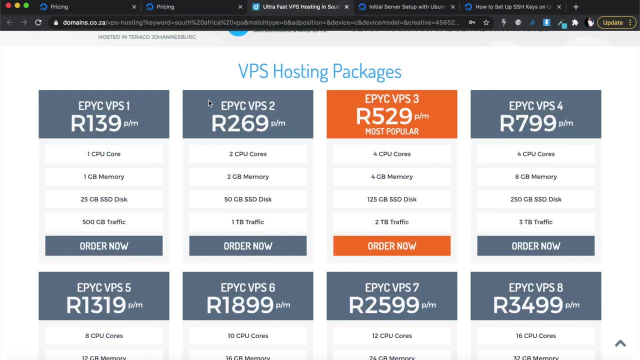 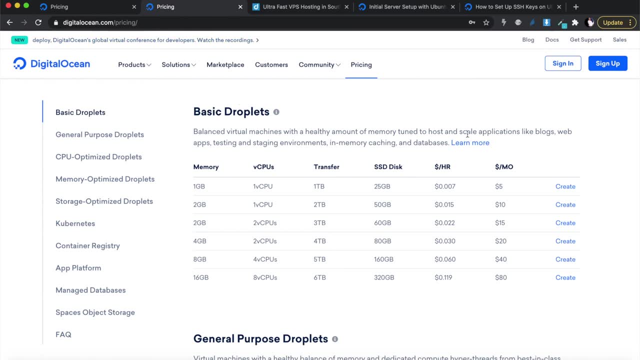 on um a digital ocean than on, uh, you know, domain social density. but then this is how you pay nine. it's also a little bit more expensive because on digital ocean you're paying just five dollars, which is about 86 rand, 80 rand. the initial ocean deal is better, but but the reason why i would 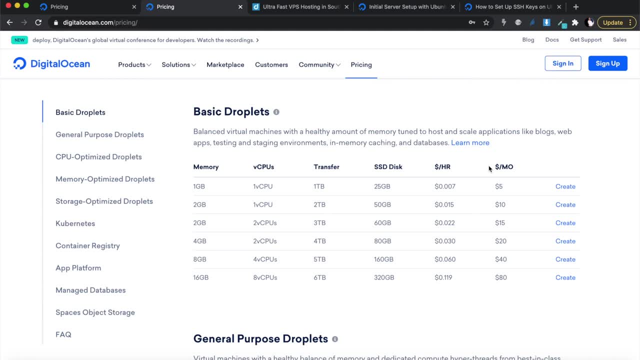 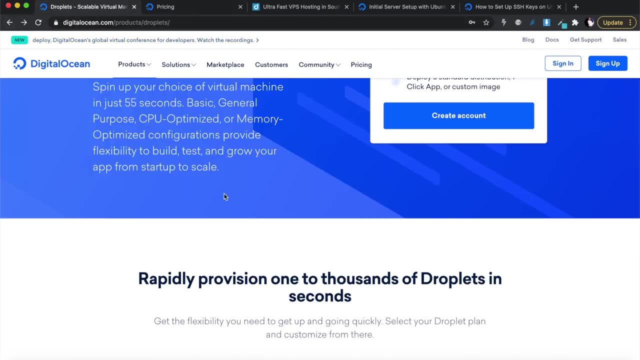 still use domains to see that, even if it was more expensive. is that digital ocean is based way? i mean, if you look at there, um, let's just go back here and look at the digital ocean. it's based on server location. uh, there are several. okay, their servers are based in the us. um, they're based um. 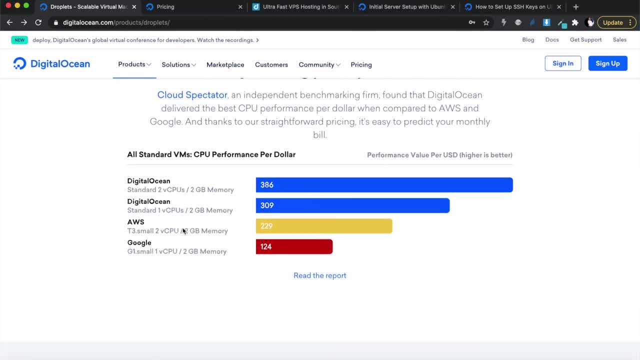 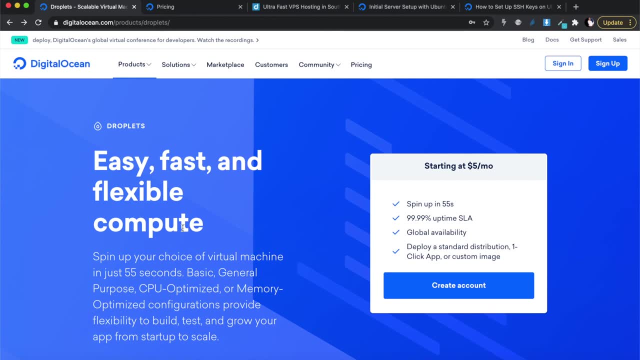 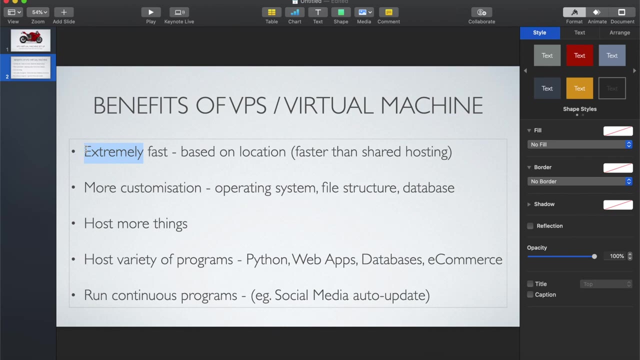 let's scroll down here. um, they're based on- okay, you can't see it here. you'll see it when you're selecting your vps machine. they're basically here. they're based in europe. they're far, far away. so it actually offsets one of the reasons why you want to use a vps machine. it will not be extremely fast. 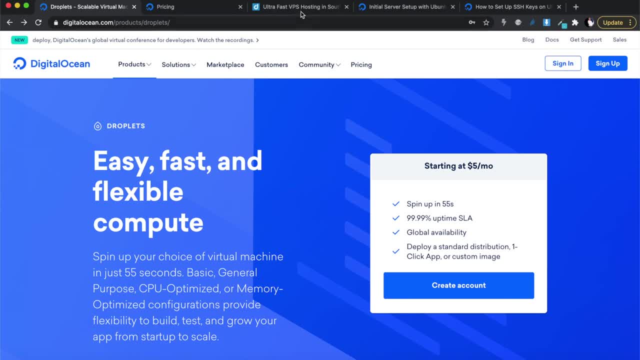 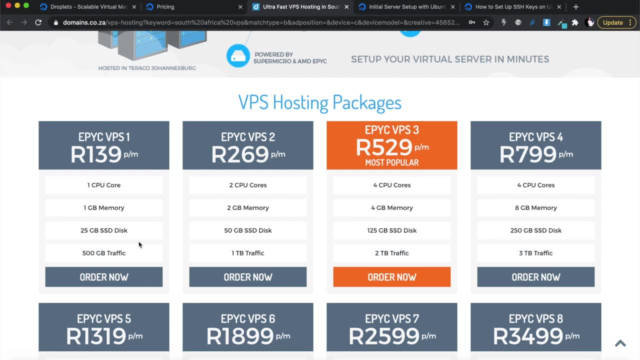 because of the location, but the south african vps and i've used it is extremely fast. so if you, if you want to optimize speed and you want to build a website and um, you focus on this here- you want your speed to be as fast as possible. actually, you're better. 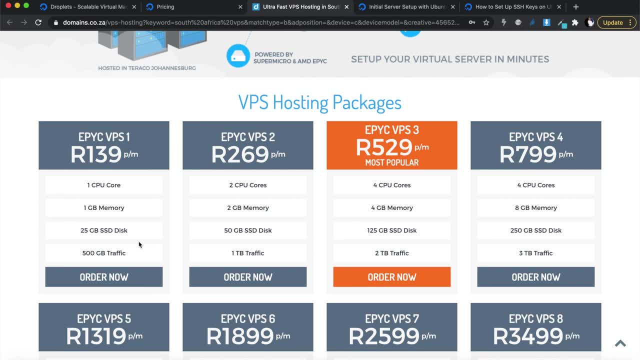 off hosting of a vps than a normal share hosting. and then you want a local vps. you don't want to work with digital ocean or you know any other cloud-based platforms that are not based in south africa. they will not be faster than the south african based ones. in johanna's book, then, um so 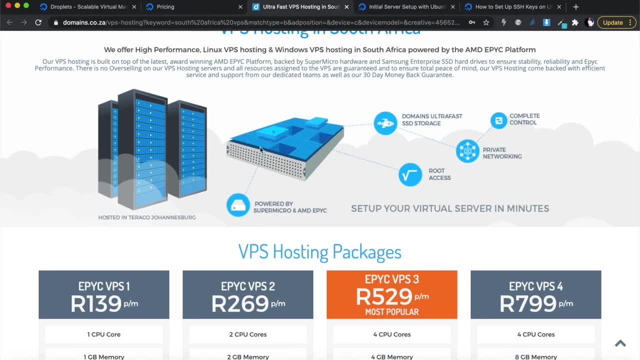 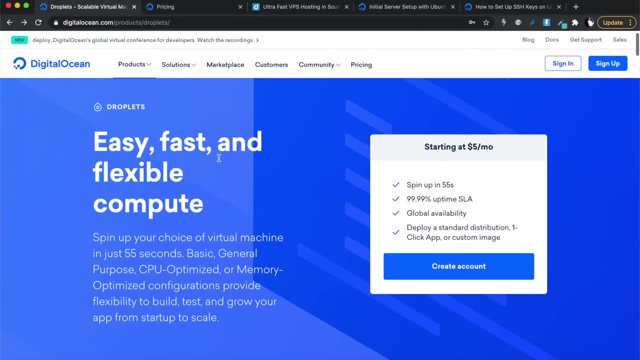 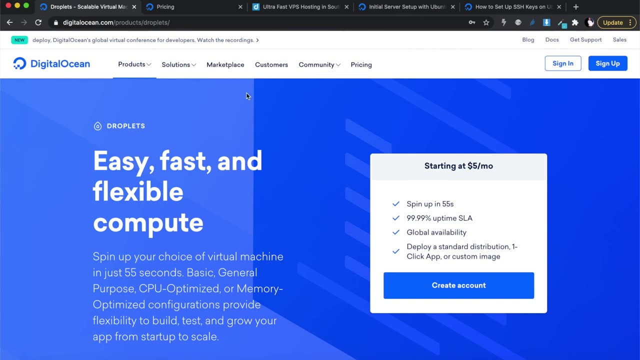 it's up to you which one you want to go for, but the setup process is going to be similar um whichever one you choose. so let's do the setup for um. let's do the setup for um- digital ocean and droplet, and the reason why i'm going to go for digital ocean is that, um, they 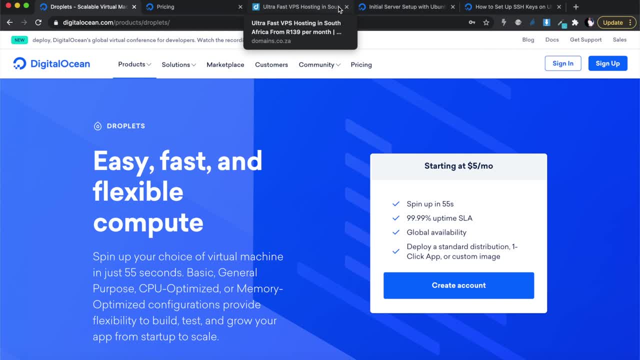 have amazing tutorials online showing you how to do a lot of these things that i'm gonna be taking you through. i'm actually going to be going through a digital ocean tutorial myself as i'm showing you this, because once you're done with this video, you can take the link that i'm 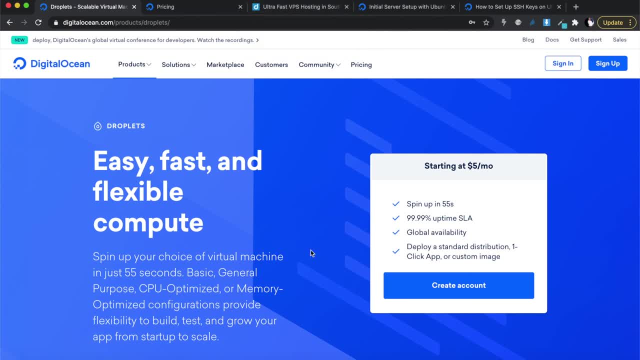 going to give to you and in your own time, because the tutorials are very well written and they're constantly revised to make sure that they're up to date. you can actually go through that written tutorial yourself in your own private time and go through the points and make sure you don't. 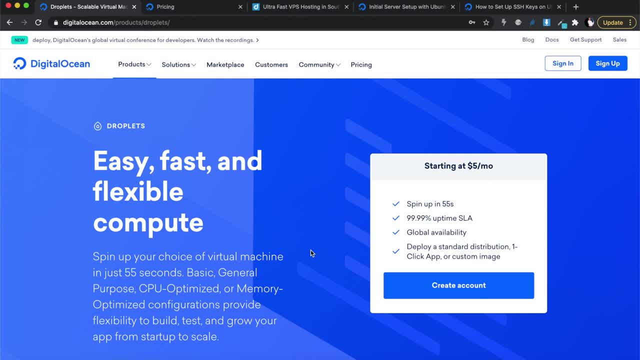 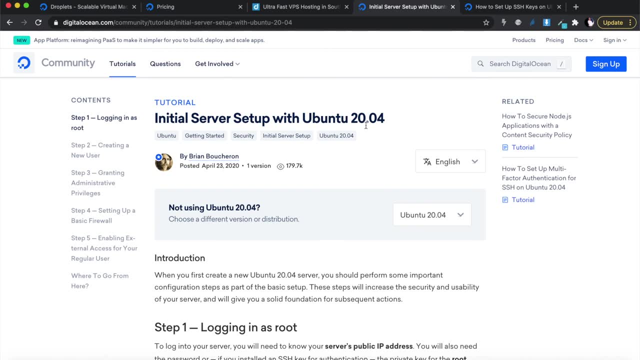 miss anything, and then you will be able to do exactly what i did here today. so the first tutorial that we're going to go through is this one here that says initial server setup with the and um. if you look at the tutorial that i will link here below, um on the, as you start to read it. 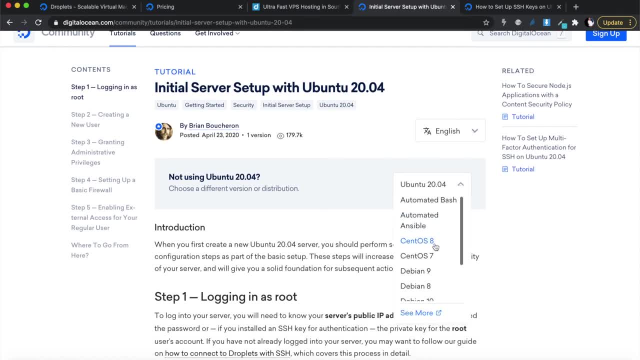 if you're not using ubuntu 20.4 um you you can choose whatever operating system that you have actually installed in your droplet and um on the drop down menu. so if you're using ubuntu 16 or 18 or deviant 10- whatever, you could select it down here, and if you click and say you're using deviant, 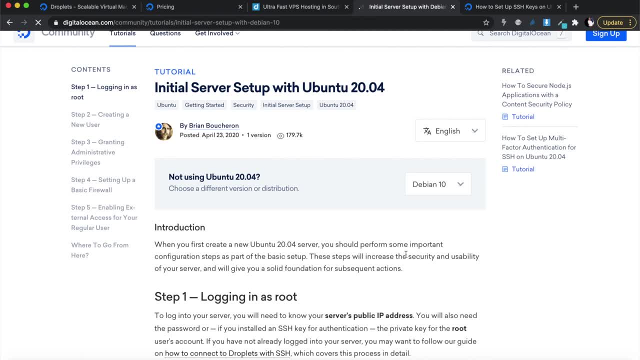 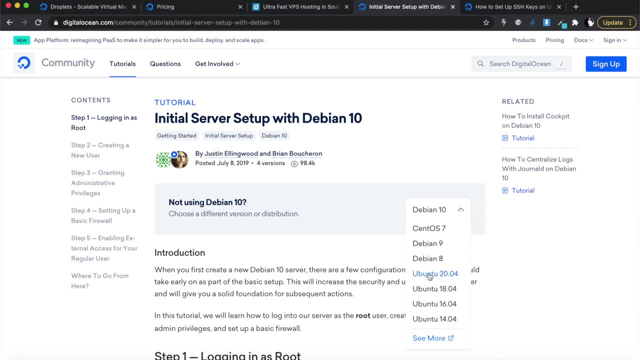 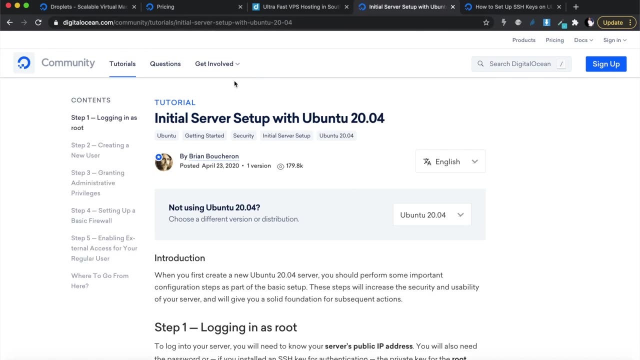 10, the tutorial will change and take you to the tutorial for deviant 10 setup. you understand so really well written. but we're going to install ubuntu 20.4, right? so we're going to go back to that, and it's going to take us back to the ubuntu 20.04 tutorial, and so let's just go through the 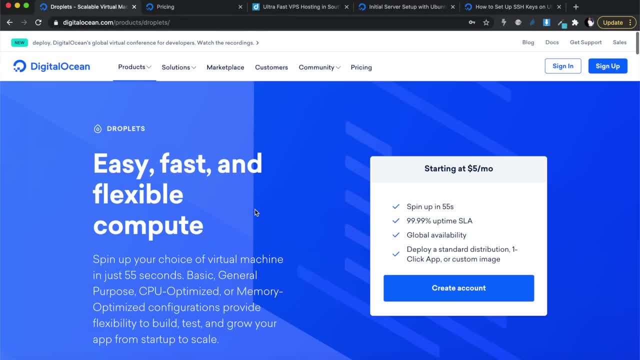 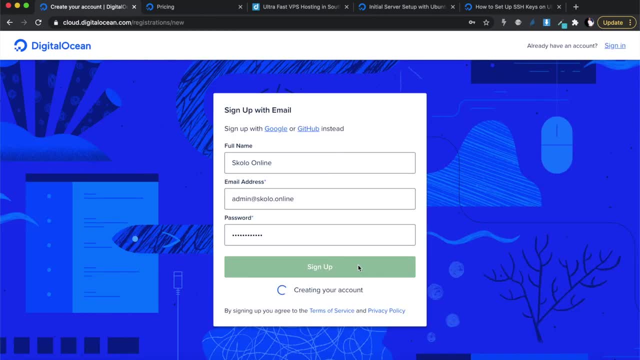 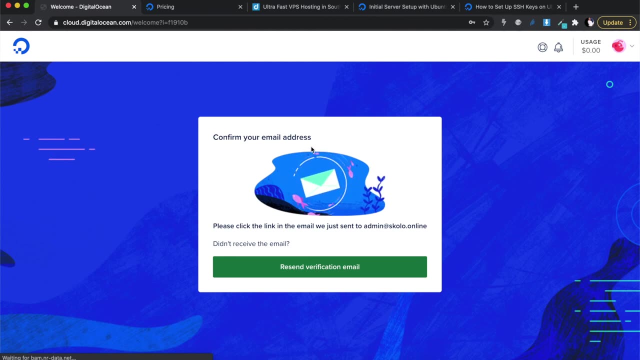 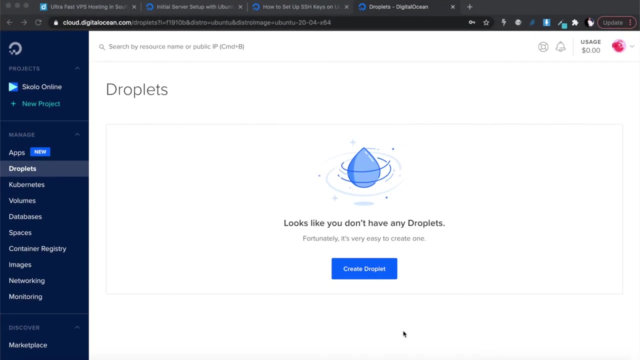 process of purchasing a digital ocean droplet. so i'm going to say: create an account. all right, when we reach this stage we will need to go to our email and confirm. so let me just do that quickly. so, once you have confirmed your email address, just go back and log into your account and um. 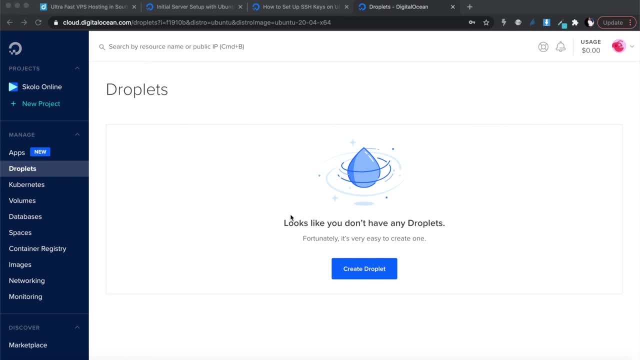 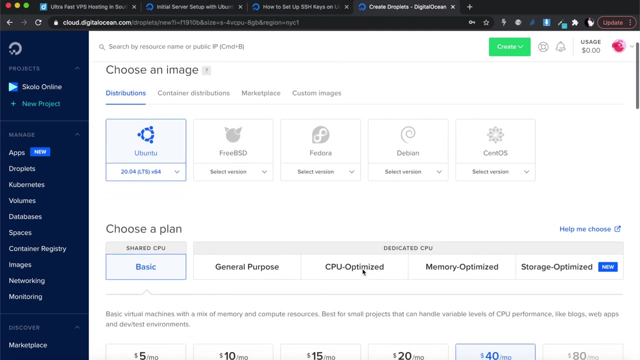 go under droplets and you will see there that you currently don't have any droplets, so we're going to start creating a new droplet from scratch, so just click on create a droplet. we are going to work with ubuntu, okay, but you could pick any operating system that you like. 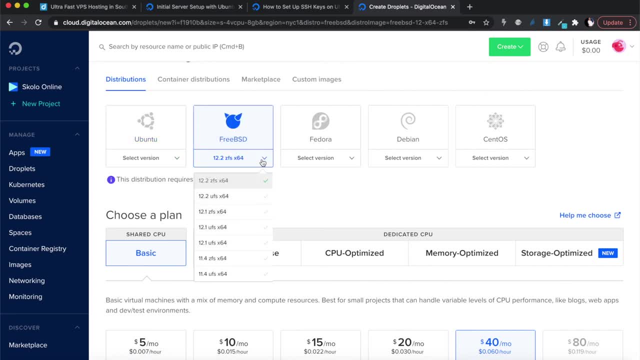 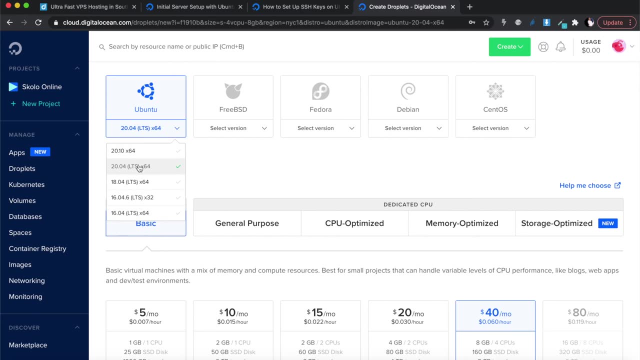 over there and on the drop down menu you can pick the version of the operating system. so, for example, we're going to pick ubuntu, but you can pick ubuntu in a different version, whatever version you like, from 16 all the way to 20 times 64.. so we're going to leave it at this one, okay, and we're 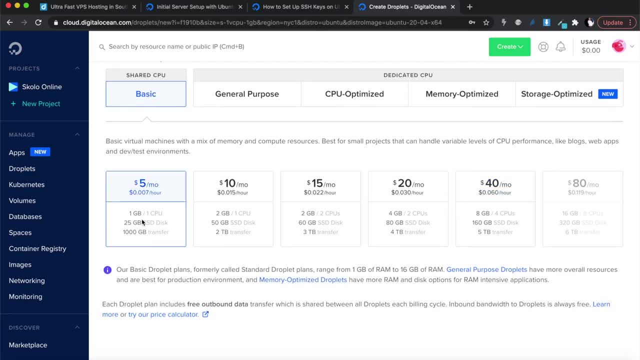 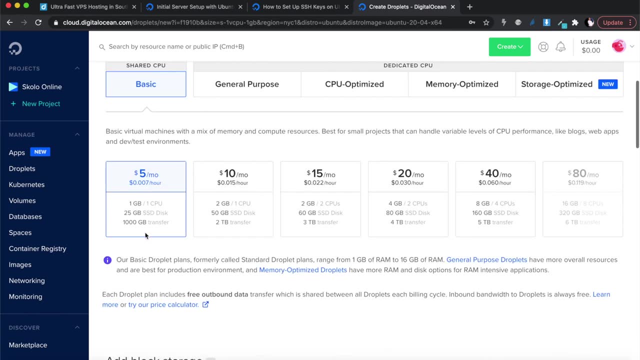 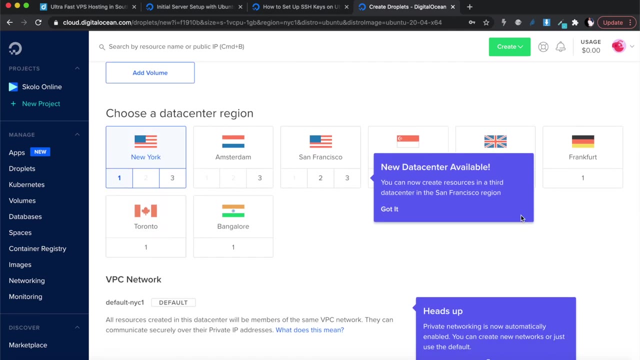 going to go with the basic plan and we're going to go with the one that is a five dollar plan, and just click on that, all right. all right. so basically, um, this five dollar plan is the cheapest one and um, that's what we're going to go for, right, then? these are all the different data centers that you can. 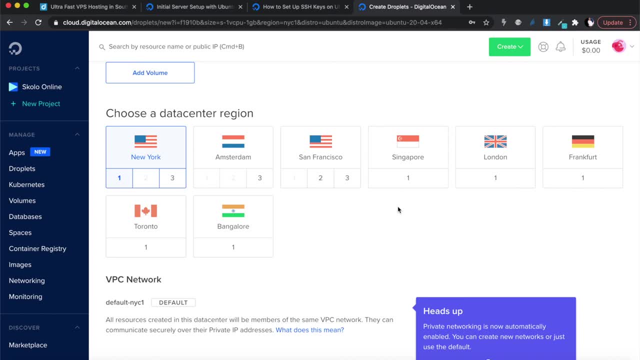 work with, and this is what i was talking about when i was saying that it's very important when your droplet is located. when it comes to speed, all right, the south african vps hosting services might be a little bit more expensive if you look at domains, but it's going to be much faster because 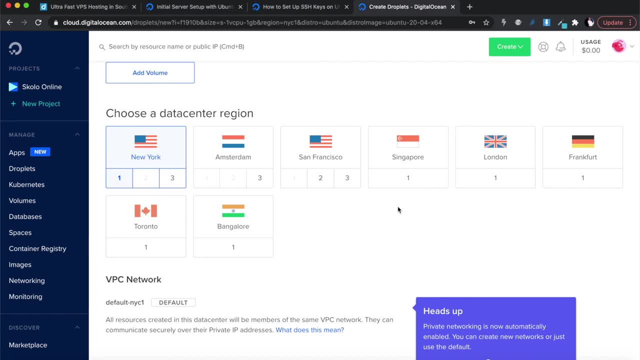 the data servers are located right here in johannesburg. going to work with a data server that is overseas? you're going to um. it's going to be a little bit slower, but not too slow. it also depends on what you're trying to achieve with your droplet. so in 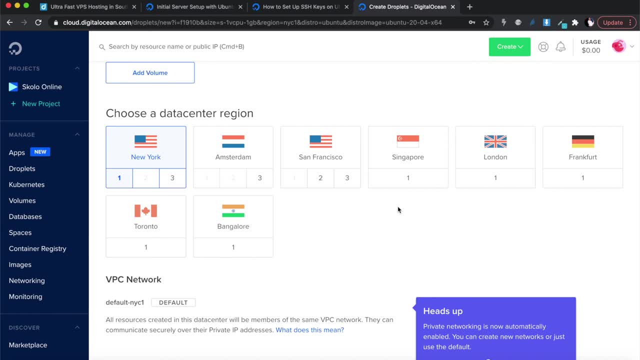 my case, i just want to build a droplet and we're going to run some python programs on it, things like updating twitter posts, sending myself emails automatically, automating some tasks which we're going to go through in this scholar online course. i'm definitely going to um, doesn't matter where. 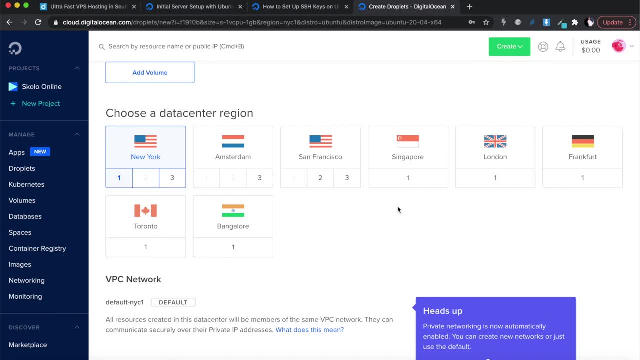 the data center is located. speed is not important, but i do not like to work with data centers of the us because of the legislation. then if you base your data, your data center in the us, it means you are governed by the rules of that country, so your data is governed by the rules of that country and 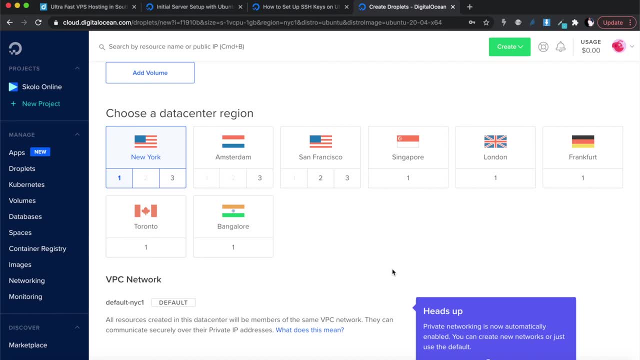 they can cease and desist your data, your information and you need to be aware of the rules of the country of where you are posting information. and i don't have time to figure out what are the rules and because i'm not doing anything majorly big but i still don't like to host in the us, i'm going to 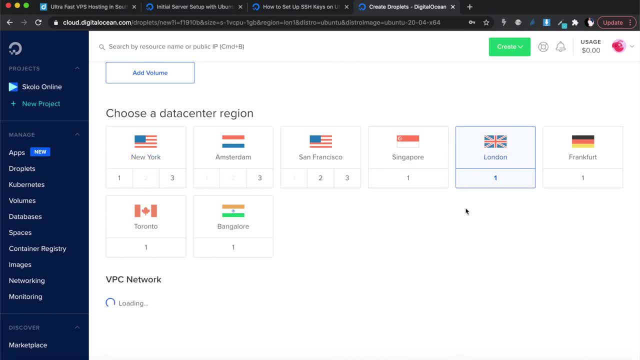 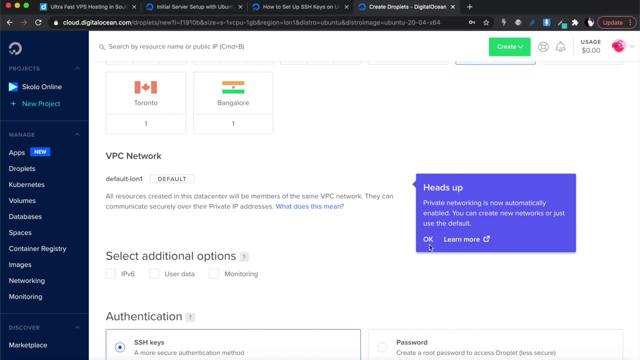 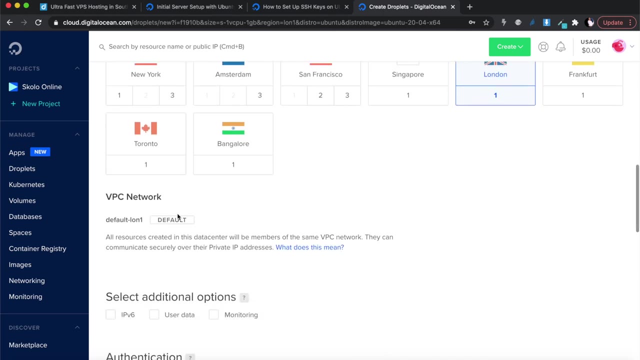 either go for singapore or london, but actually i think london is better, so um, closer to me, and i also like the fact that we are almost in a similar time zone. um, with london then, um. so once you've done that, you're gonna see the vpc network, the default, that's fine. 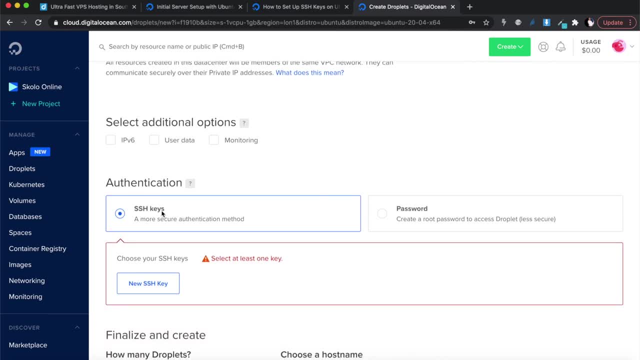 select additional options. no, we're not gonna do that, so you have two. when you get here, you have two options, and this is very, very important, and please take note of this. um, you can either go for ssh keys or you can create a password. all right, a password is. 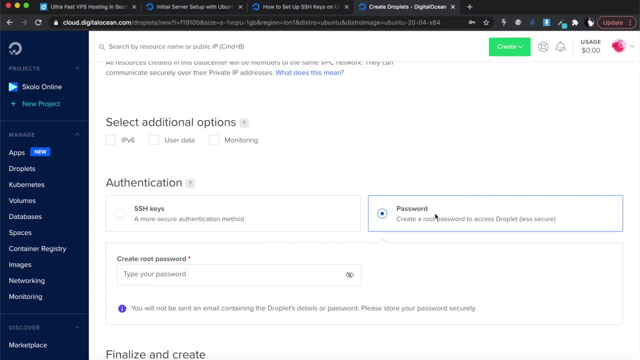 definitely less secure and i do not recommend that you do it. please do not go for the password option, because a password option is easy to crack. all somebody needs to do is to learn your password and, just like that, they have access to be PS a machine. all right, but you can also select SSH keys and and then work. 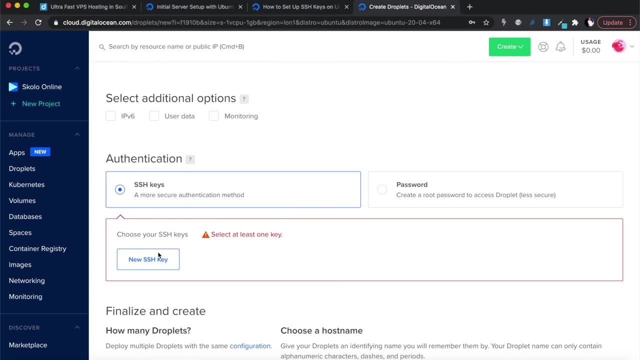 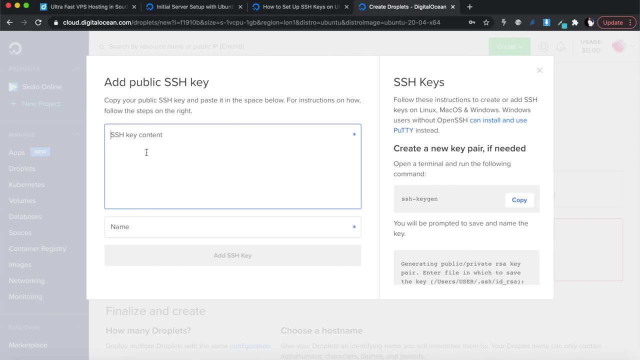 with an SSH key. so let's look at the SSH keys. so if you select SSH keys, you would have to submit a new SSH key and then you need to, you know, put in the key content. the SSH keys has two to two parts. they have a public key and a 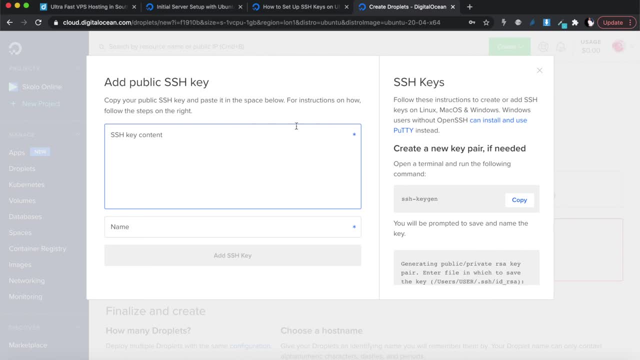 private key. all right, so what you can do is that you can what you call follow the this instruction to create SSH keys on Linux. all right, create a new key page needed, open the terminal and run the following command: okay, so you can go to your terminal and run this command and then you're gonna get a key that you can. 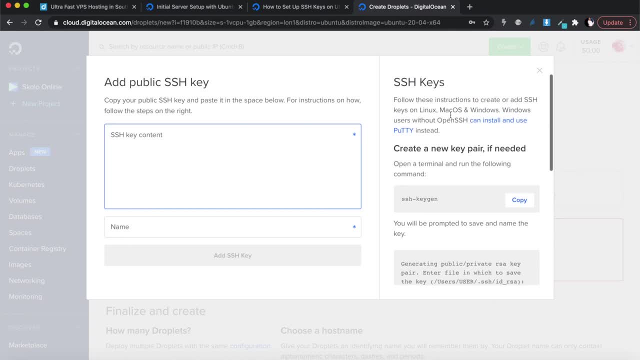 then copy and paste somewhere else and do it that way. but I don't want to do it because I really have an SSH key on my terminal and I don't want to create one here because then it's going to be a clash with my other SSH key. so I'm going to 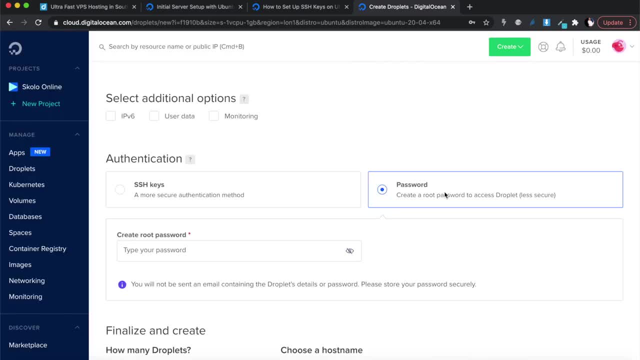 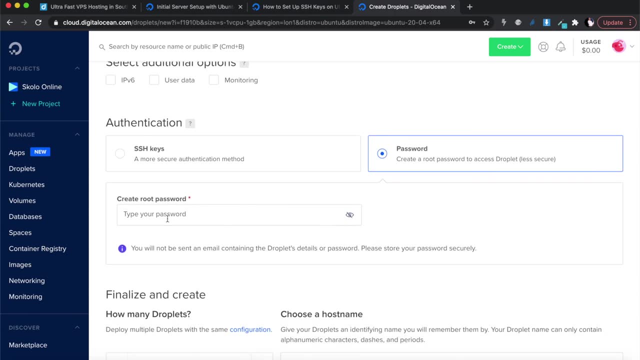 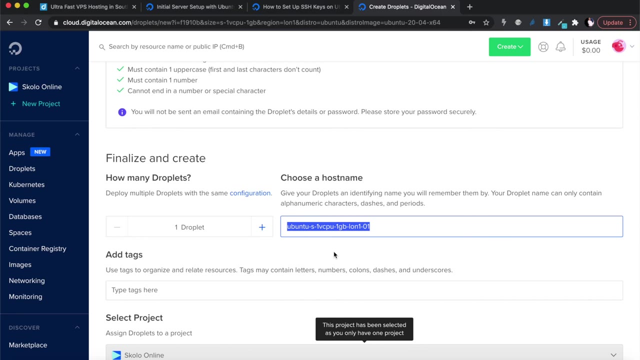 actually go back to the password option, but keep in mind, you actually want the SSH option, so let's go for the password off, all right. once you've done that, you can choose the name of what or your machine, what you want to call it. all right, so I want to call it. 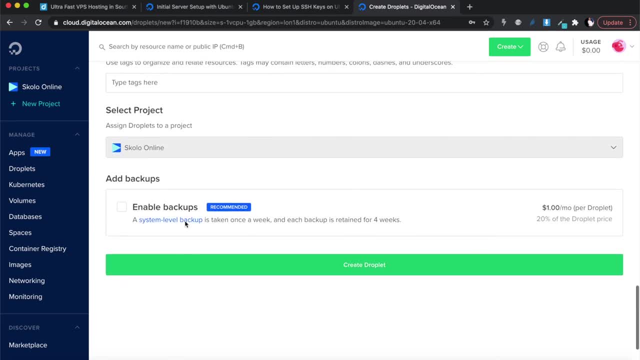 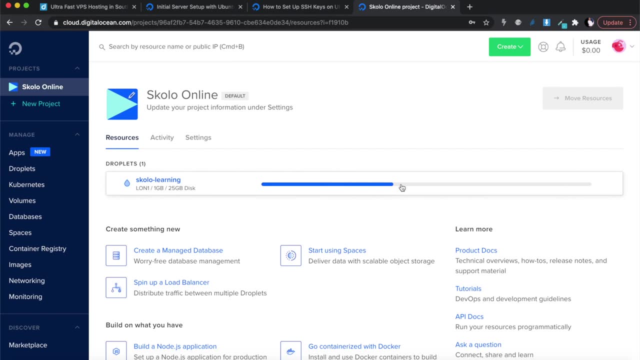 and I don't want to do backups at all, mind about that- and then you're going to clean up the job, it right? so it's working, working, working, working, working. alright, once it's finished working, take note of your IP, right, we can just copy that. all right, then you can go to your terminal, any terminal window, and you can. 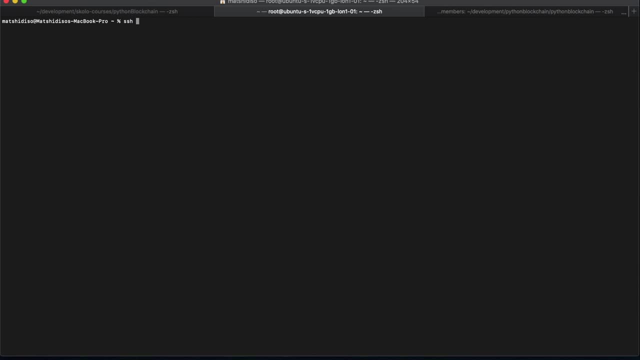 Just type SSH, right root at that, all right, your ip- and press enter, all right. so it's going to ask you: do you trust this machine? you want to connect with them? yes, i do, all right. and then you have to enter the password. this is your root password that you created. so every time you log into your machine, 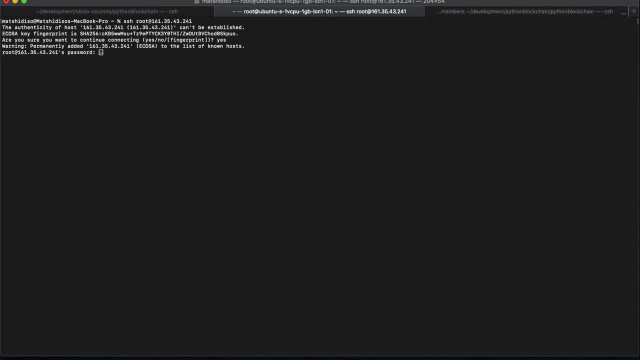 you are entering the password there, you go all right and you can see that you are root at scholar. okay, so we are now inside the vps machine and we can run command. we can do anything we want inside the vps machine, but i actually want to follow this tutorial that we have here. 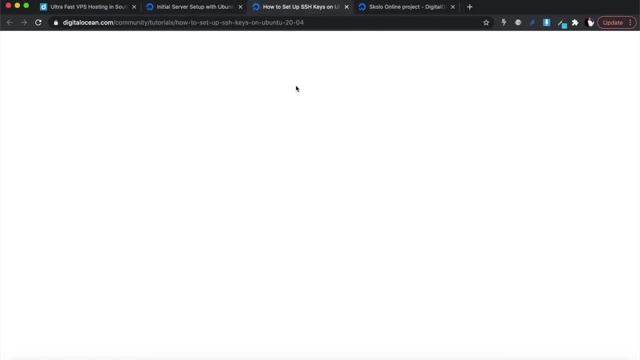 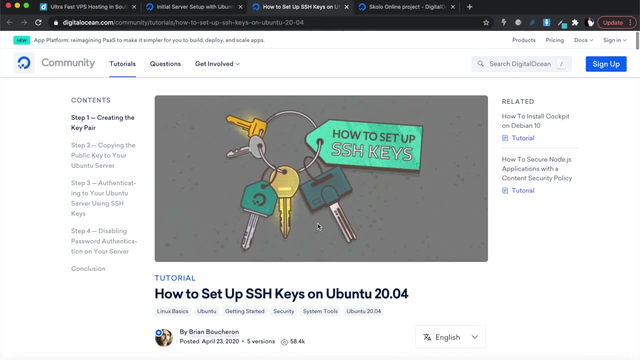 um initial server setup with the boot and we have also the tutorial for setting up ssh keys. i'm going to also keep this um for you and i'll link it on the description below and you can follow this. and please do set up the ssh keys before you do anything else, especially if you're going to do anything. 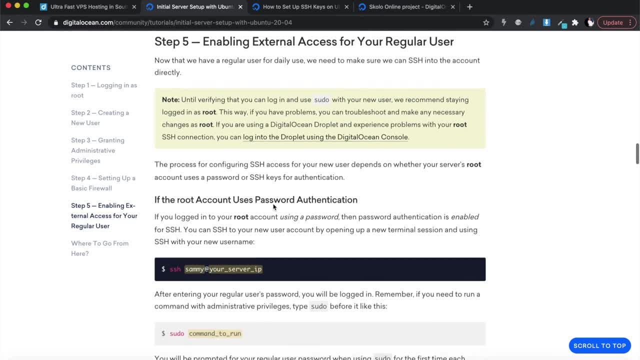 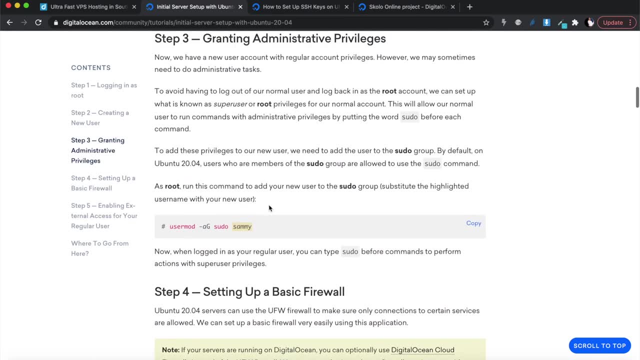 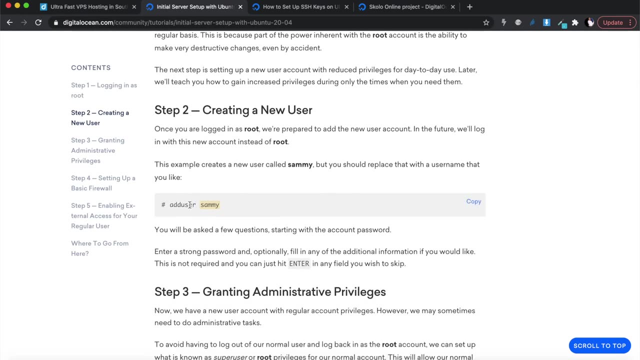 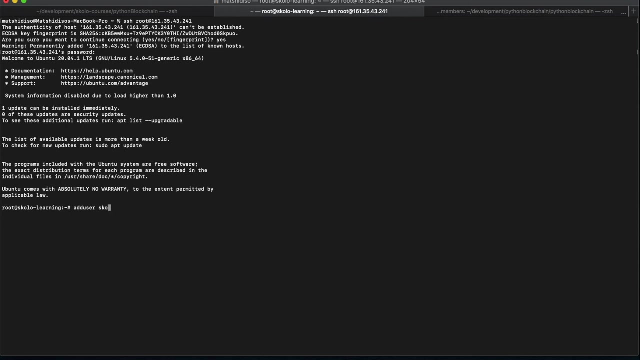 important, but for what we're doing, we can work off the passwords. okay, so let's try this tutorial. all right, so i've already logged in at my ip and then i want to add a user. okay, add user called scholar, the user password. let me type the password. 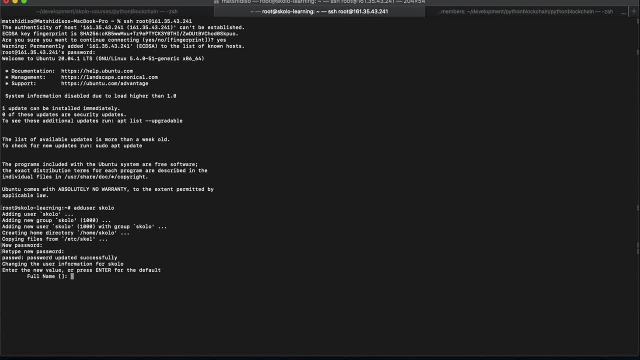 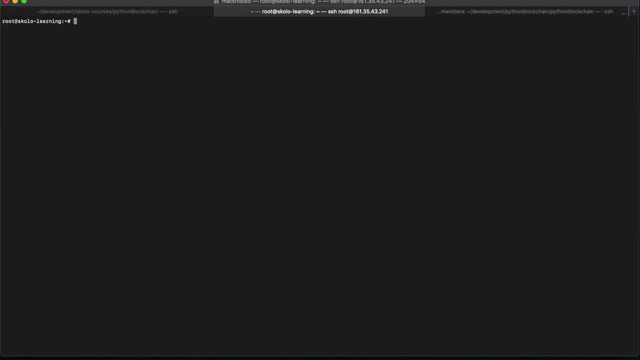 all right, my full name is room number, phone data. it's correct. yes, all right, so that's done. we'll set up a new user. and then what we're going to do after setting up the new user, we're going to modify the user privileges of our news. okay, so let's just do that. 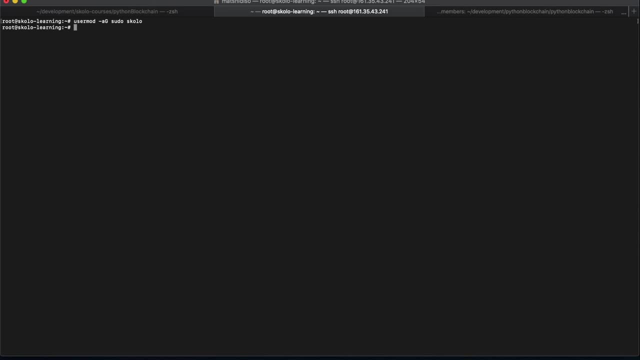 awesome. so user scholar should now have pseudo privileges. okay, and let's test this quickly. so let's exit. exit and try logging in as ssh scroller at our ip address. so this is our ip address. i just copy it and paste it there again. all right, and let's enter in our password again.